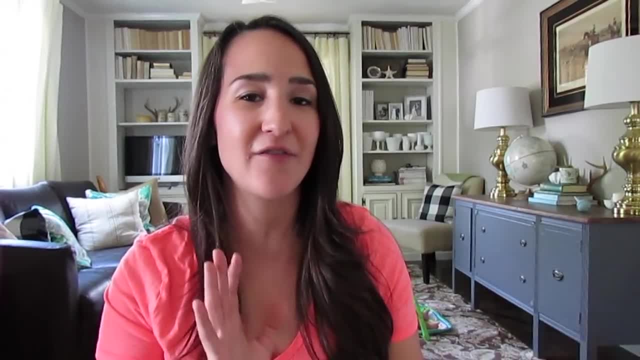 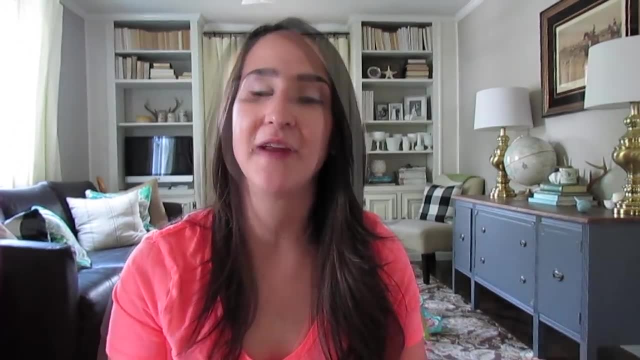 hold. The cabinet is actually pretty generous, so she has all of her favorite Peppa Pigs and princesses and a couple of games that she loves to play with in there, So that's what we keep in the console table. Our built in bookshelves in the back also have some. 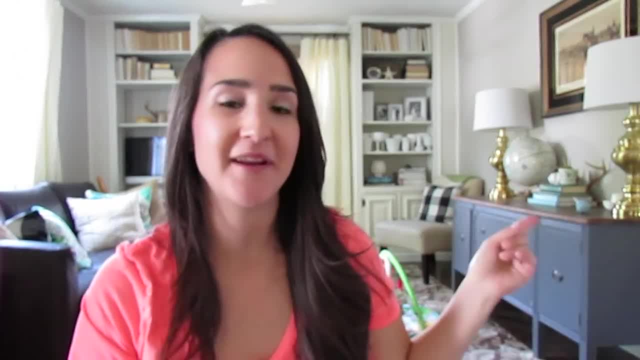 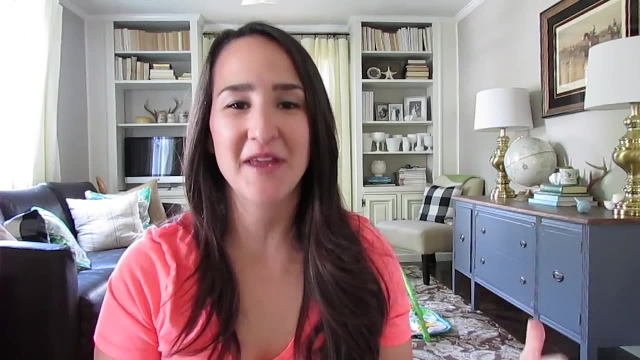 toys that we keep in there And then we keep our little toys that Evie and I have in the shelves in the back- also hide toys. The cabinet on the right side has books, tons of books. on the bottom overflow books because Evie has tons of books in her bedroom, but we keep. 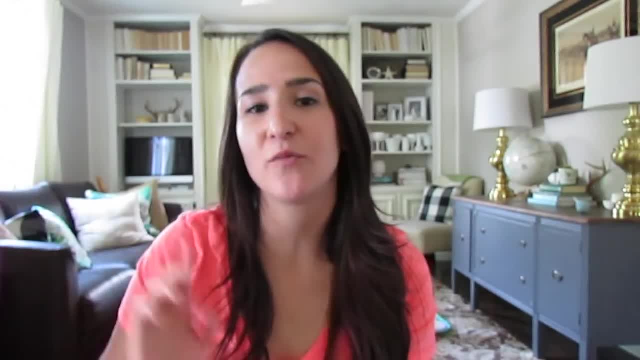 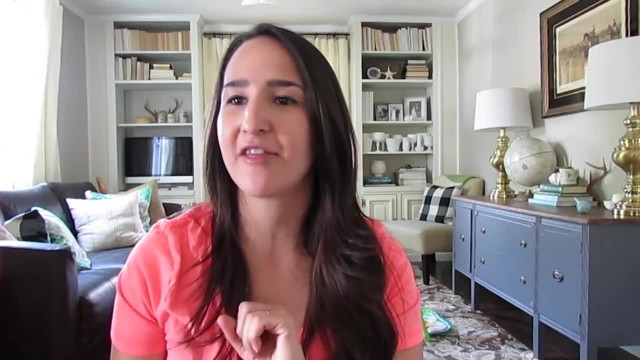 some more in here for her. In the cabinet on the left built-in, we keep Evie's Mega Blocks for building, which she loves to do all the time, and a tea set and a little chair cover that my sister made her And those are basically her favorite toys. so those are. 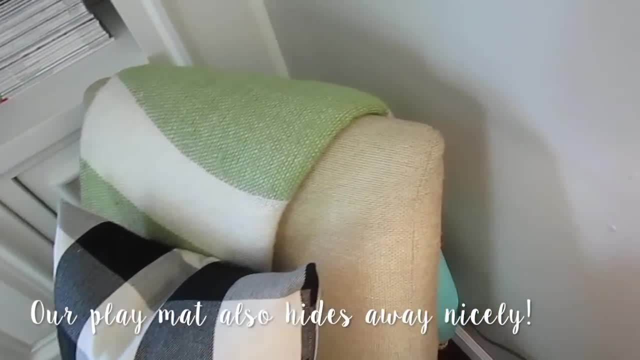 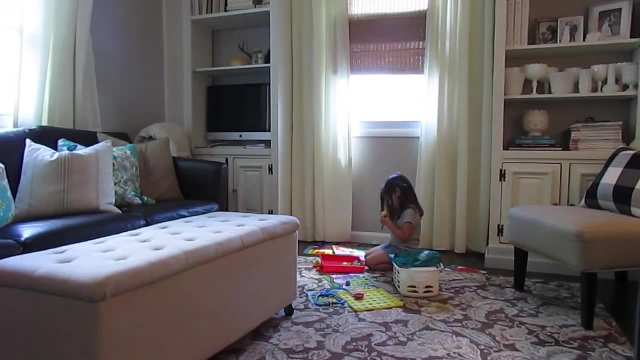 the ones that get to stay in the living room, and we easily hide them behind cabinets and doors. And then my next favorite piece of organization in the living room is the ottoman. So of course, this is functional for us because we can put our feet up on it. I change, Lara. 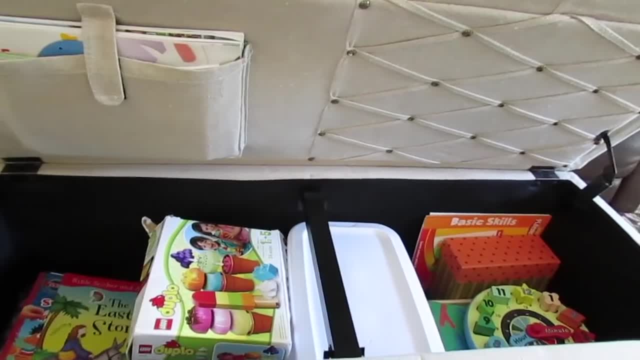 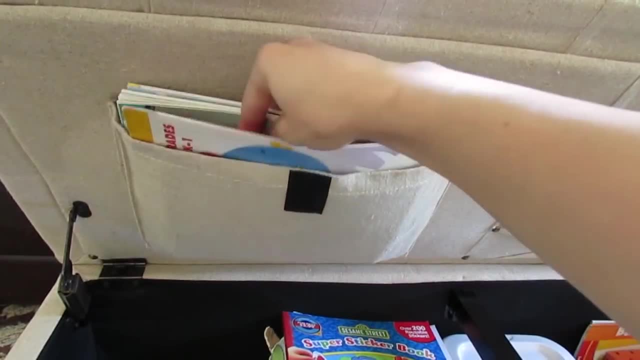 on it all the time on a blanket, But inside is all of Evie's learning materials- so educational, like games and wooden manipulatives and cards and little workbooks and all sorts of things like that. all live in that ottoman. I do have some more in our closet, but the bulk of it. 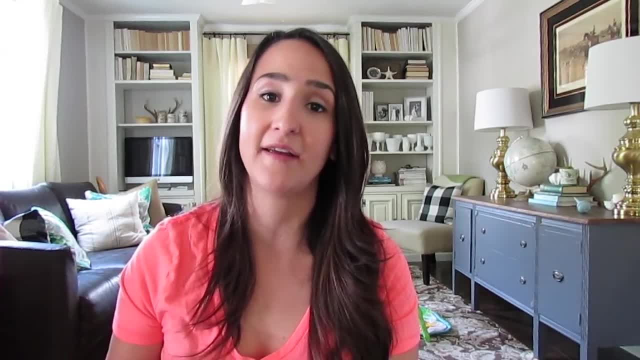 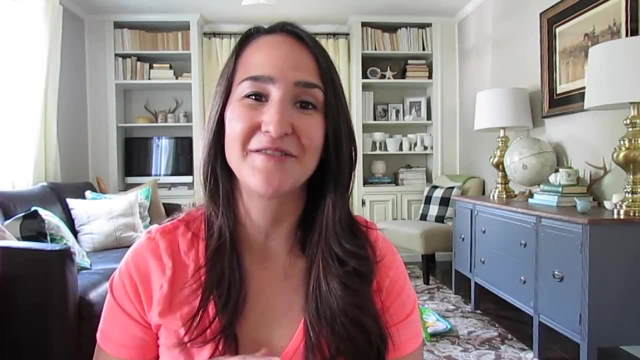 does live in that ottoman and those are things that she is allowed to just go ahead and get into and use anytime she wants play with them. I don't keep like markers or crayons in there, because we don't want to- you know, set her up for a disaster, But we do keep. 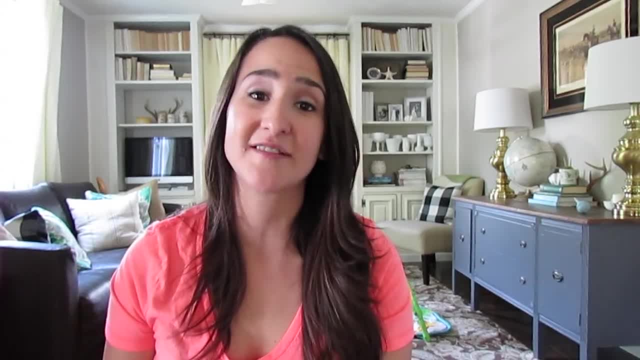 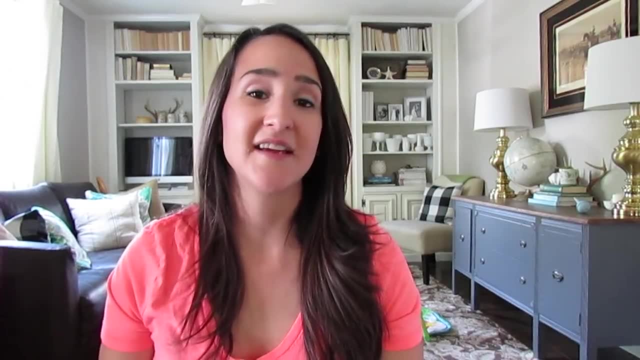 it all in there. It's great that she can take it out and play with it and then, when it's all done, we put it in. you close the lid and the living room is back to clean and beautiful And that's it. That's pretty much all the kid stuff that we keep in the living room. 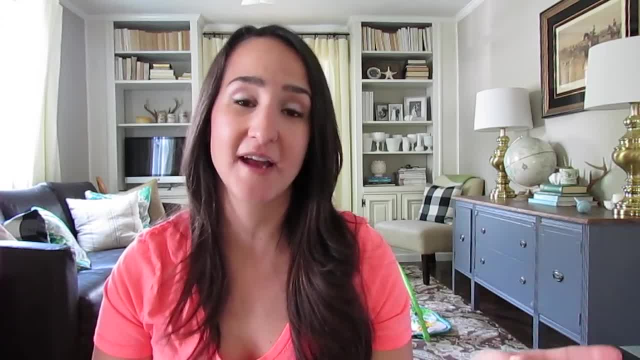 Everything else either goes in Evie's bedroom, and I did do a video about how I organized her bedroom which I will post in the description box below. So if you have any questions or questions, I will link to if you're interested. And we do also have a basement playroom where 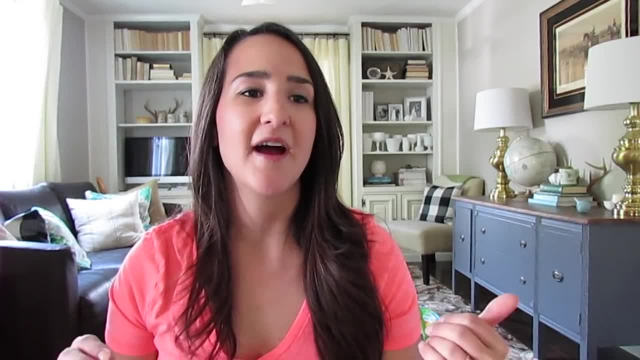 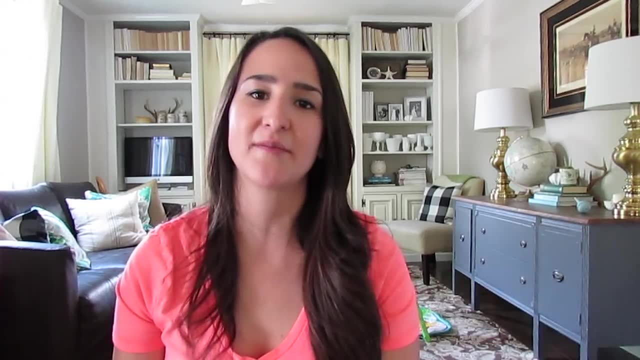 we play down there every now and then. There isn't a ton down there, but if there's ever anything that she doesn't seem to be that interested in anymore, sometimes I'll rotate out with things that are in the basement. We'll bring something up and bring something.